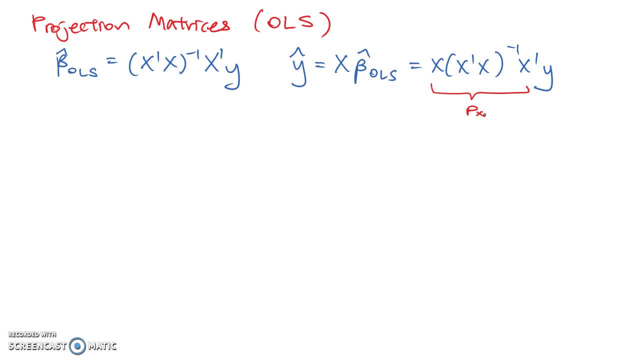 px times y. So the projected values of y are simply equal to the projection matrix times the original value of y. So, in other words, px is simply shorthand for the projection matrix. Let's illustrate this with a simple example. Okay, let's have a situation where the x matrix is equal to 0,, 0,, 1,, 1.. 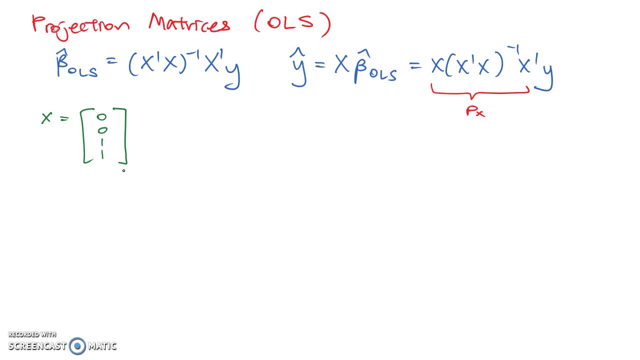 And in this case, x tells us a person's work status, whether someone works or not. So in this case, we have a data set of four people. The first two people, The first two people, don't work because their value is 0. 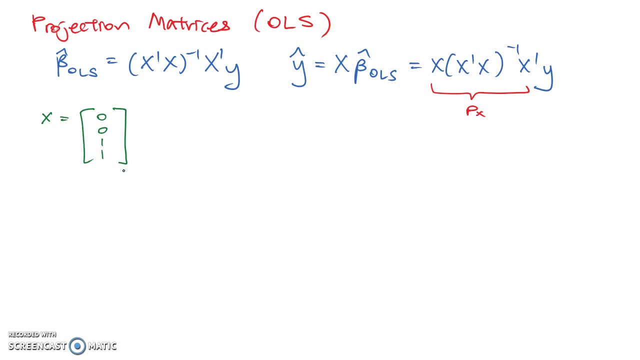 And the third and fourth people work, and hence their value is 1.. And you also have data on their wages. So let the y vector be their wages And if you don't work, obviously your wage is 0.. And for the people that work, for the sake of an example, 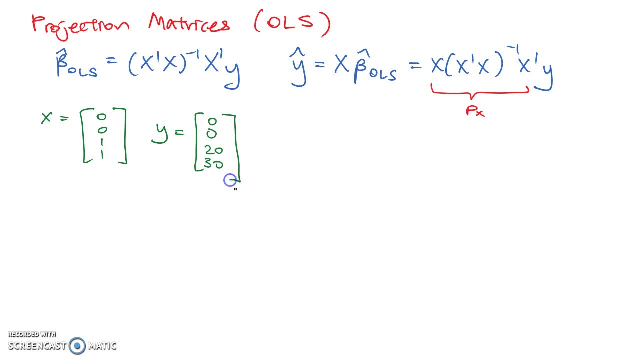 let's just say that their wages are 20 and 30 respectively for the third and fourth person. So let's calculate what the projection matrix will be In this case. we have 0,, 0,, 1,, 1.. And then we need the x prime, x inverse, which will be equal to this. 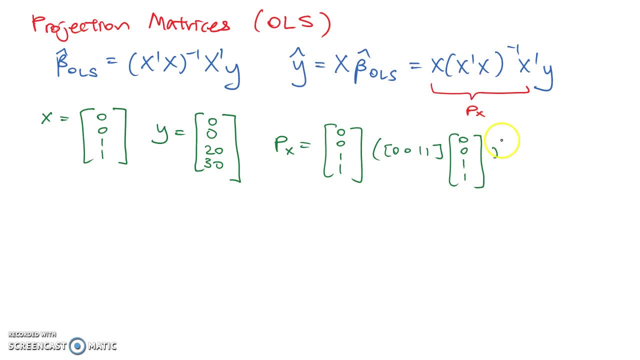 So 0, 0,, 1, 1.. It will be 0, 0, 1,, 1, x. And then we need the x prime x inverse. In this case, we have x prime x- 0, 0, 1, 1, x. 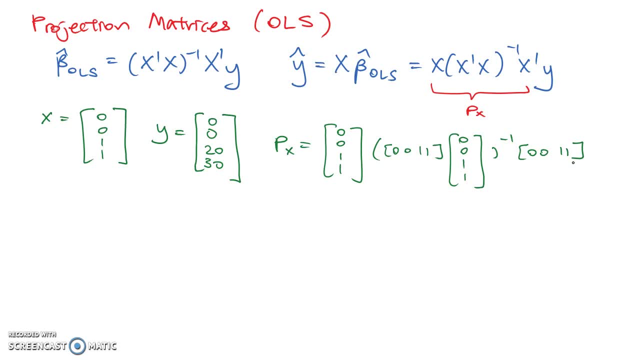 This is equal to 4, 0,, 1,, 1, 1.. So this is theinverse And this is further multiplied by 0, 0,, 1,, 1, x, x, prime. And if you were to work everything out, 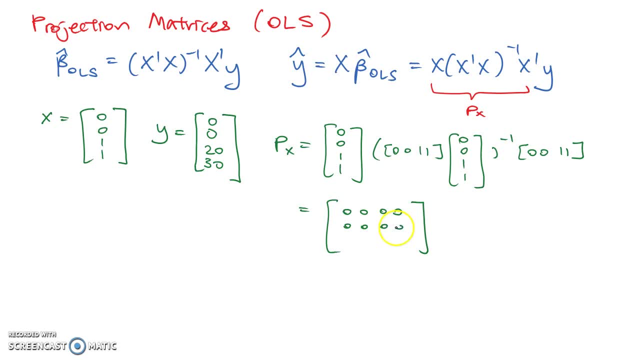 you will find that this is equal to a 4 x- 4 matrix, where you have The first, last two rows, have some ones, and the whole thing is multiplied by half. you, you can check it using an online matrix calculator, so no, so notice that p x- y is equal to half times this entire. 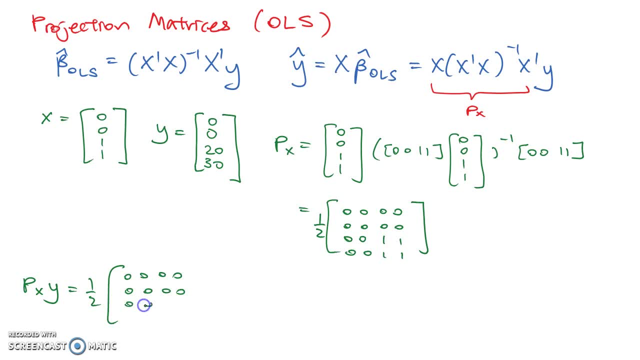 matrix and then we we further multiply it by 0, 0, 20, 30, and when you do the matrix multiplication you find that this is equal to 0, 0, 25, 25, and recall this four times: one matrix with with values of 0 and 25 is your predicted values of of y. in other words, for these two people. 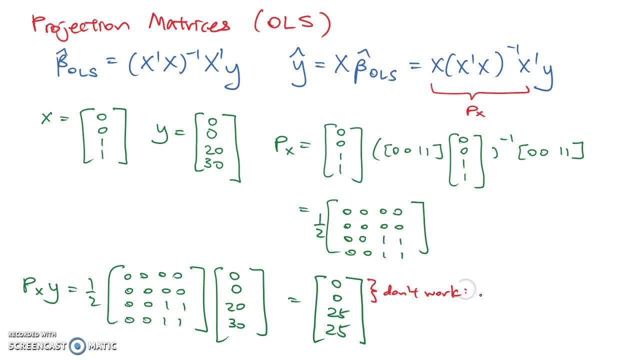 that don't work, their predicted, which is zero, or their projected, which is zero for those that work. they're pretty. they're predicted, which is 25.. notice that 25 is simply the average wage of the of the people that work, and in this case it makes intuitive sense, since the average wage is is 25.. in other words, if you have no 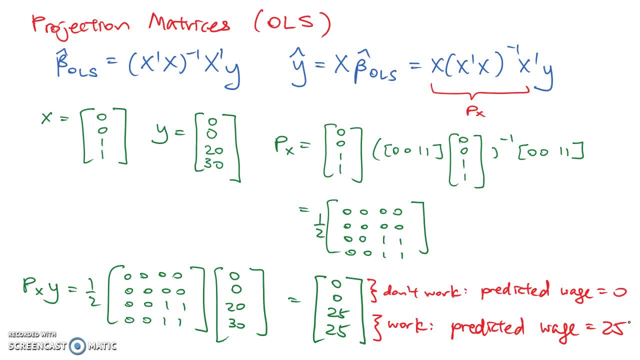 no information about someone except for for the fact that he or she works. then you'll be able to predict that the wage is 20- 25. but you can't do any better than that. notice that the notice that the y hat matrix is sim is simply a linear function of the x matrix.